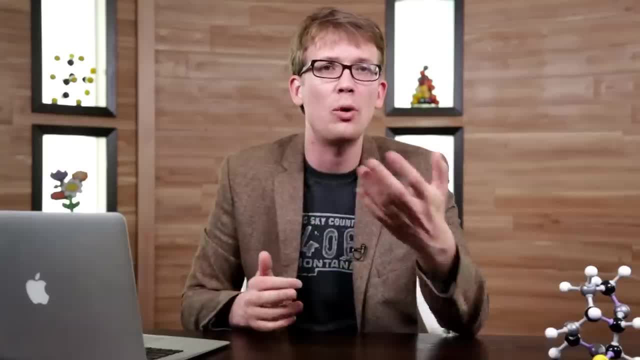 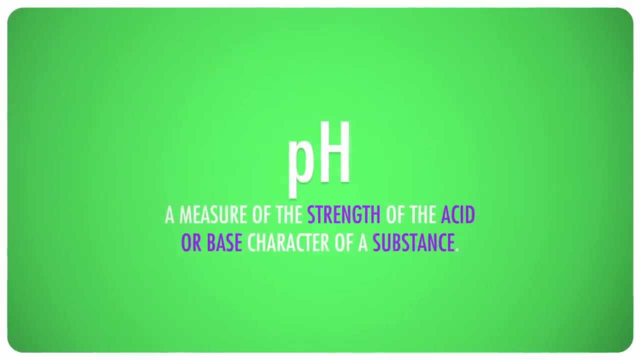 The H part is even easier. it stands for hydrogen, because hydrogen ions, or protons, are pivotal to the behavior of acids and bases, which is what pH describes. So you can think of pH as basically the power of hydrogen in a solution, the strength of 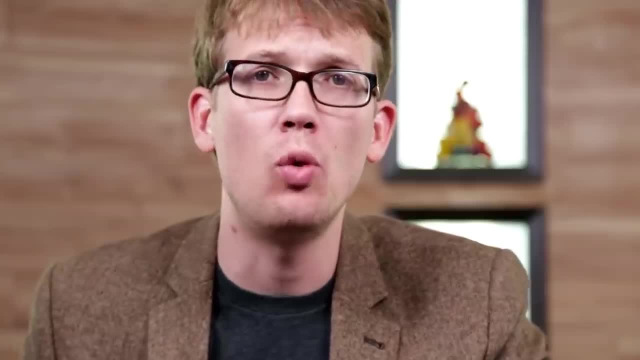 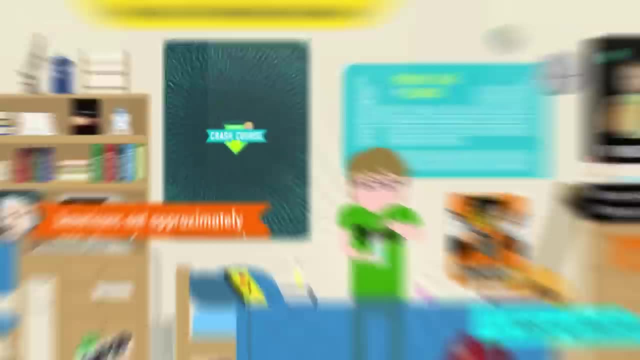 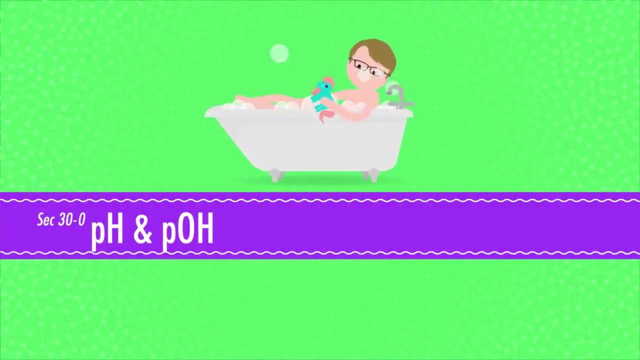 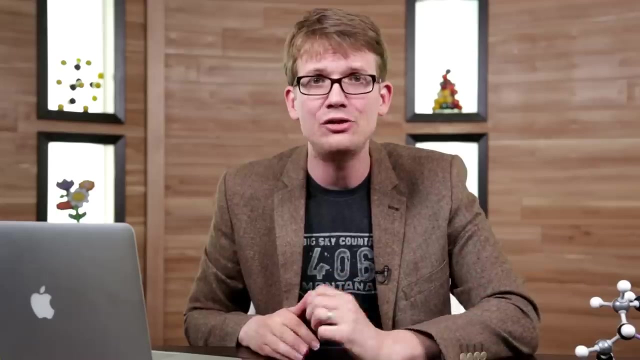 the acid or base character of a substance. And it all revolves around one very important point of focus: our old friend water. If you've been watching Crash Course Chemistry from the beginning, you've gotten the message that water is special in more ways than I can list, and pH is just one more of those. 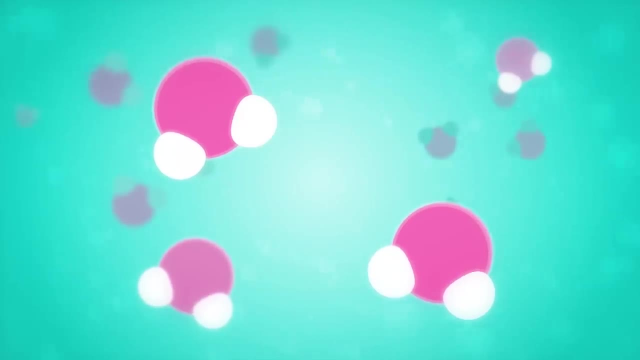 ways. We normally think of water as a perfectly neutral substance, Neither acidic nor basic, But it's not, And that's true. but, as I've mentioned before, water can also function as an acid releasing hydrogen ions, also known as protons, and as a base consuming them. 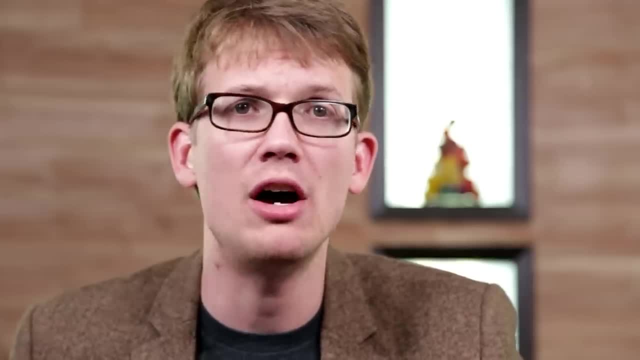 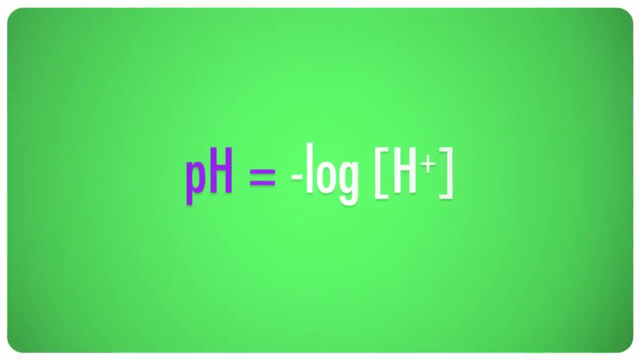 How on earth is that possible? In order to explain, we first have to understand what the pH of a substance really tells us. While chemically we say that pH represents the power of hydrogen in a solution, it's mathematically defined as the negative of the base-10 logarithm of the concentration. 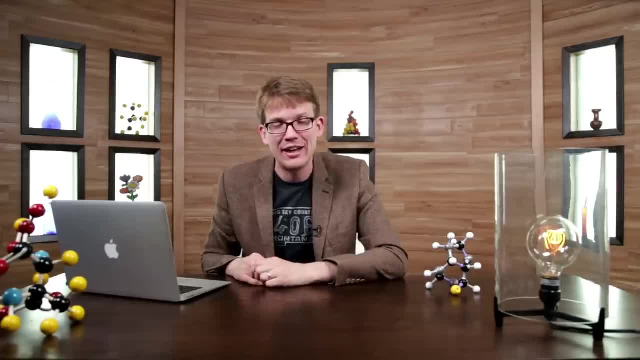 of hydrogen ions in solution. Okay, so, now that you're terrified, I'm here to explain, I'm here to help. So, yeah, logarithms can seem a little bit scary at first, but the ones that we're using here are super easy. 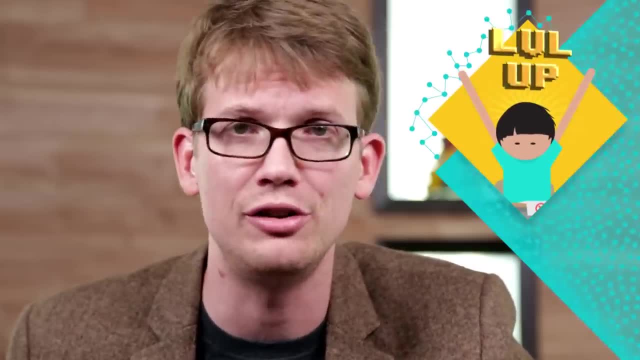 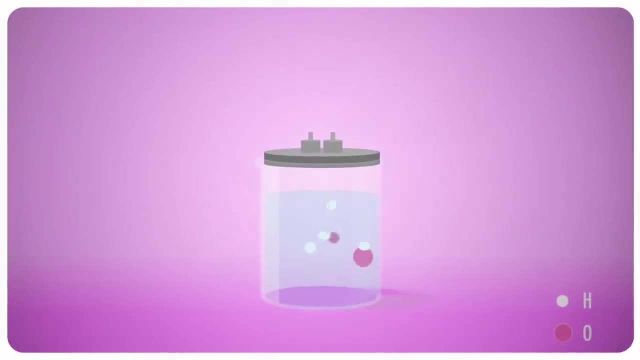 And bonus: once you get familiar with them here, it'll be that much easier to understand them in math class. So now that we've got the scary mathematical definition, let's do the simplest mathematical definition. At any given moment, there will be a certain number of hydrogen ions in solution. 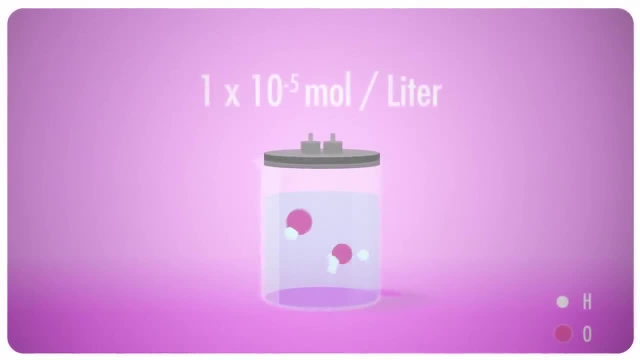 A very small number. The concentration will be a number like 1 times 10 to the negative fifth moles per liter. That negative 5 is your base-10 logarithm. Take the negative of that and you get the pH 5.. 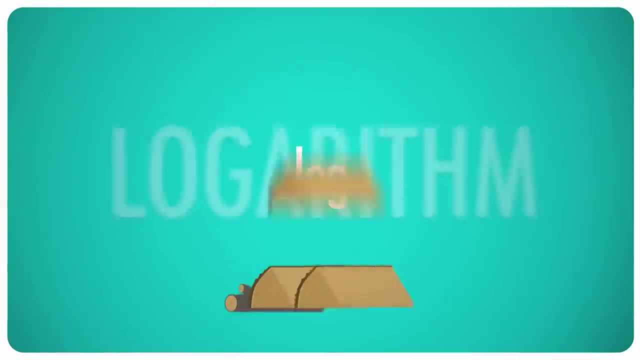 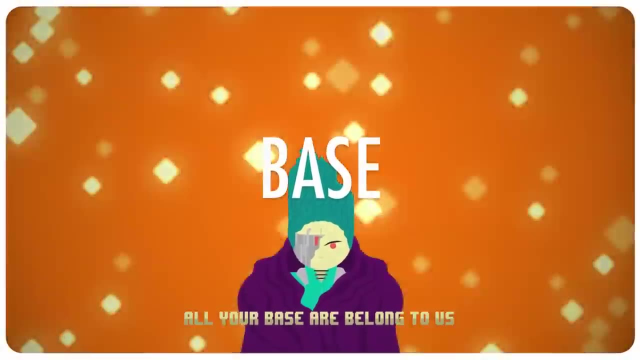 Now let's get a bit more into the weeds. The logarithm, or log, of a number is the exponent to which another number called the base must be raised to produce the target number. So for base-10 logs the base is 10.. 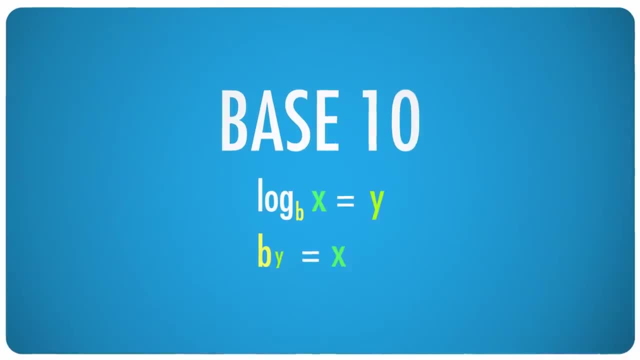 They're what we use most in chemistry and they're really easy to understand, and also what we base scientific notation on. So, as an example, the base-10 logarithm of 100 is 2, because 10 raised to the power of 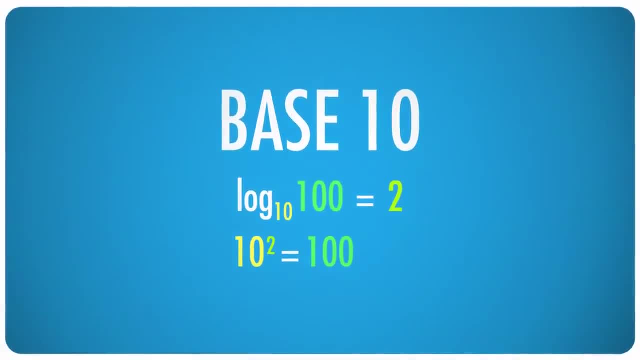 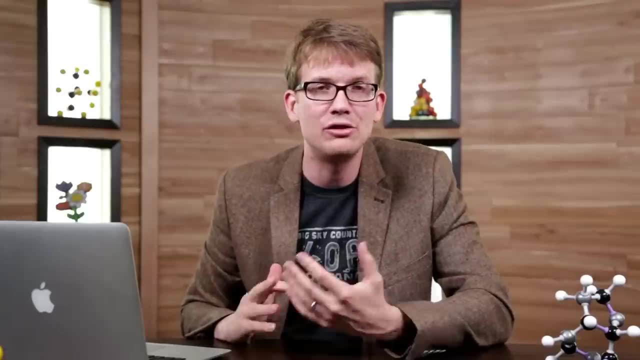 2, or 10 squared equals 100.. Base-10 logs are so common that we often lose track of them. We even leave the subscript 10 off when we write it, Like if your calculator has a log button. that's just for base-10 logs. 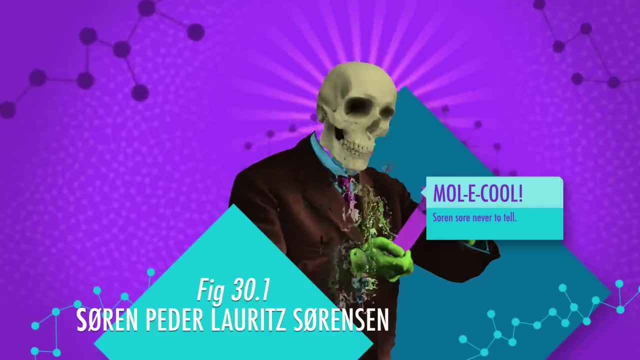 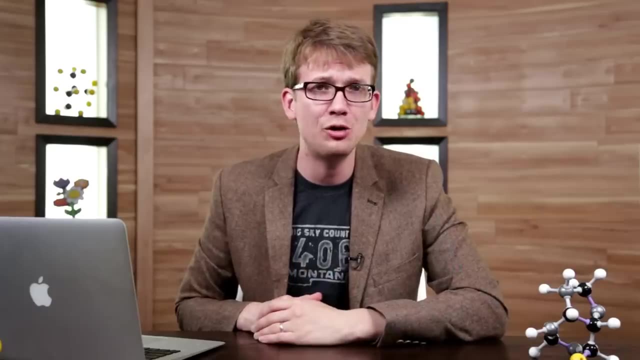 So what in the name of soren sorensen? does this have to do with face-melting acids? Well, I'm getting to that, and it all starts with water's crazy potential to act as both an acid and a base. Random changes in the tiny electrical fields around the atoms in water occasionally cause 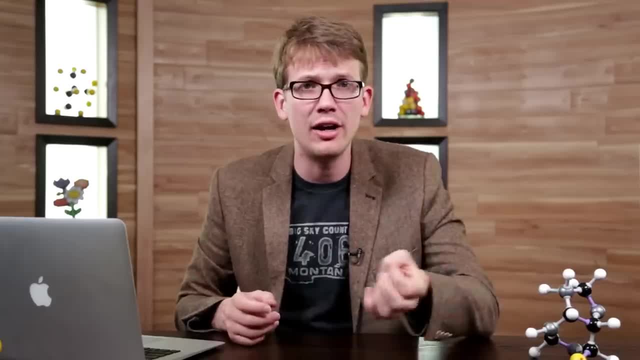 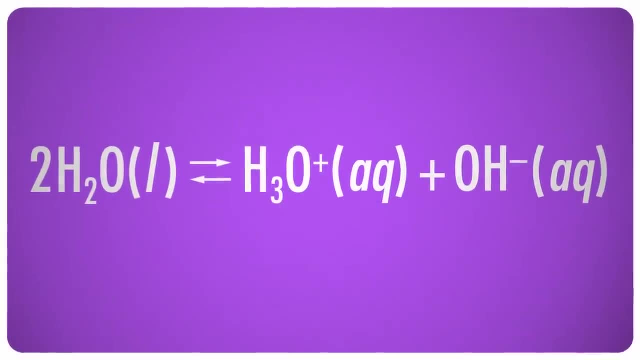 the molecule to break apart. Specifically, a hydrogen ion or proton, will break off from one molecule and attach itself to another one, Using a hydronium ion H3O+ and a hydroxide ion OH-. This is why water can act as both an acid and a base. 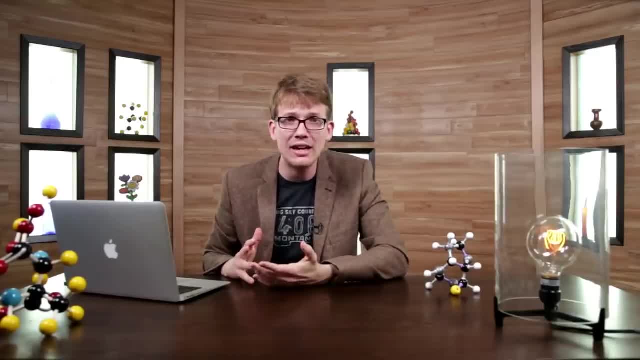 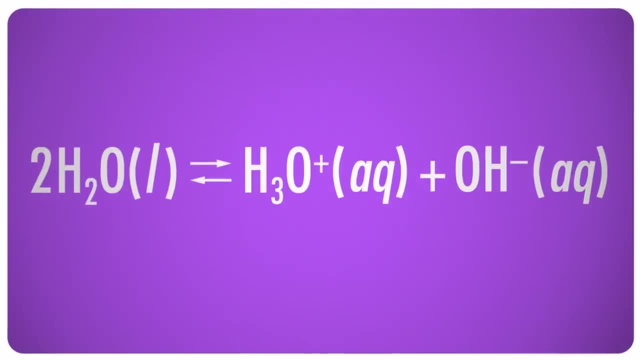 Its molecules can both release and accept protons. In this case it's only interacting with itself, but water can interact in the same way with other acids and bases. Sometimes you'll see the hydronium ion written as a simple hydrogen ion H+, allowing the 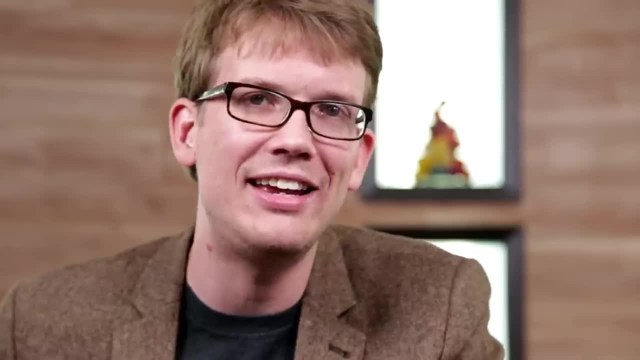 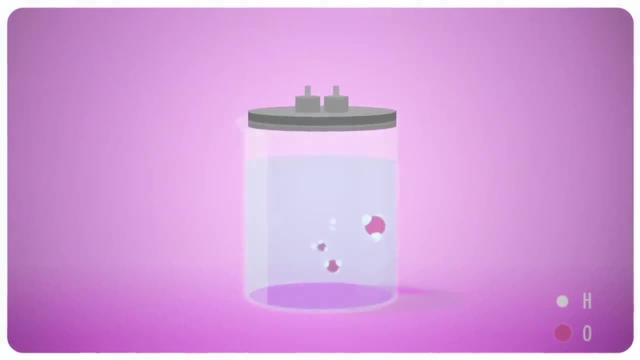 reaction to be written with only one water molecule. It's not technically accurate, but it's close enough to reality that it can be used to simplify things. If the pH is the negative log of the hydrogen ion concentration. yeah, we actually mean hydronium ion concentration. 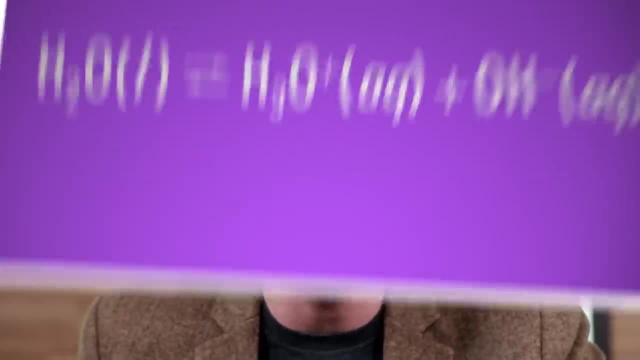 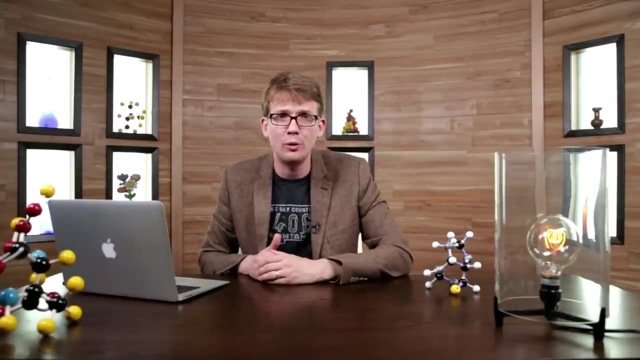 Just another thing that early scientists got a little bit wrong and now we have to live with. Anyway, this dissociation of water is a reversible reaction and in fact, the ions always reform into water within a tiny fraction of a second. But it's happening all the time, constantly in your bottle of water, in the water inside. 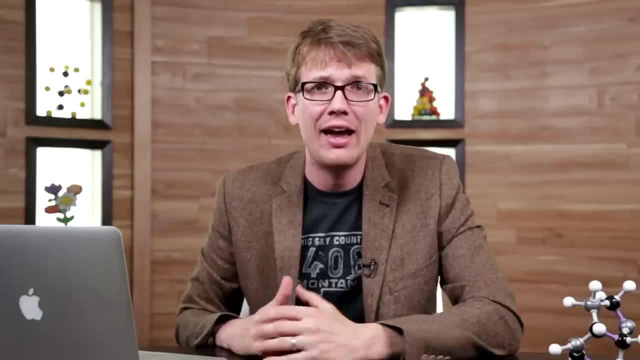 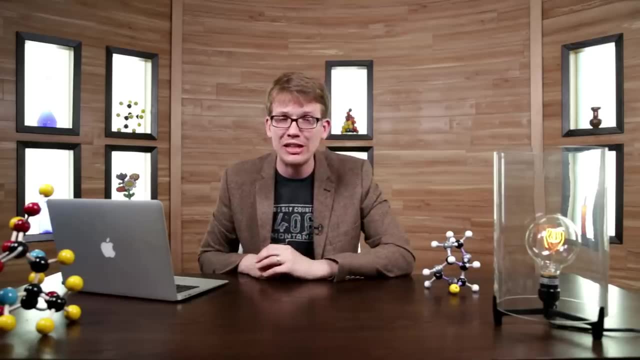 your cells and in the ocean always. However, at any given instant, only a tiny number of molecules will be released. That's why it's called a hydrogen ion. In fact, the exact number of these molecules is well-known to chemists. 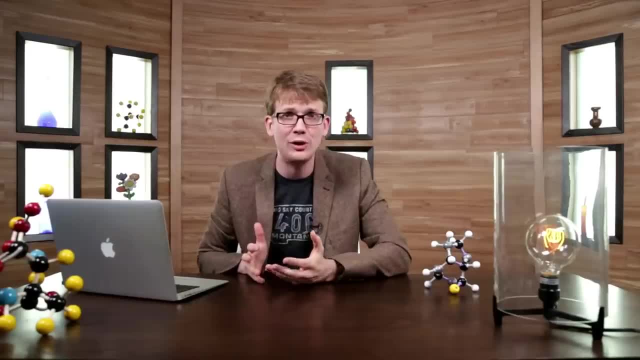 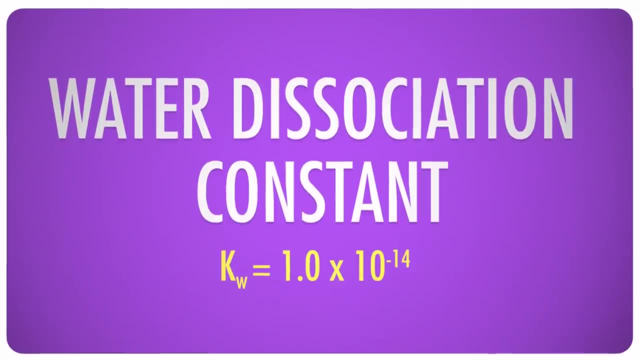 It's the equilibrium constant for this reaction and because it's such a special reaction, it has its own name. The water dissociation constant, or Kw. Kw is equal to 1.0 times 10 to the negative 14th. 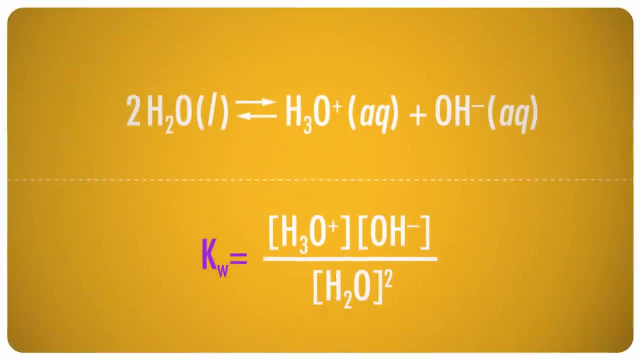 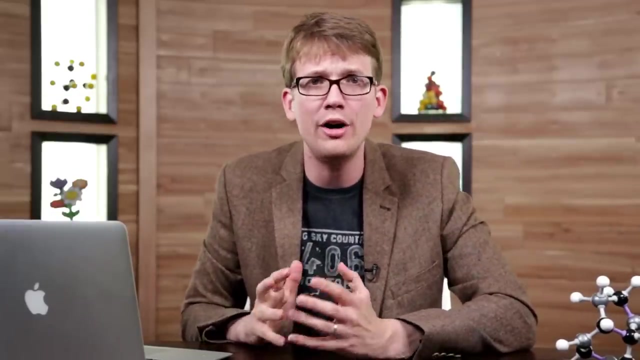 The formula for Kw is set up like any equilibrium: constant Concentrations of products over concentrations of reactants, all raised to the exponents based on the coefficients of the balanced reaction. There is, however, one difference: Because the ions represent such a tiny proportion of the total mass, the water itself is essentially. pure And pure substances, because they don't have concentrations, aren't included in equilibrium calculations. So the formula for Kw becomes simply the hydronium ion concentration times the hydroxide concentration According to the balanced equation for the dissociation of water, hydronium and hydroxide. 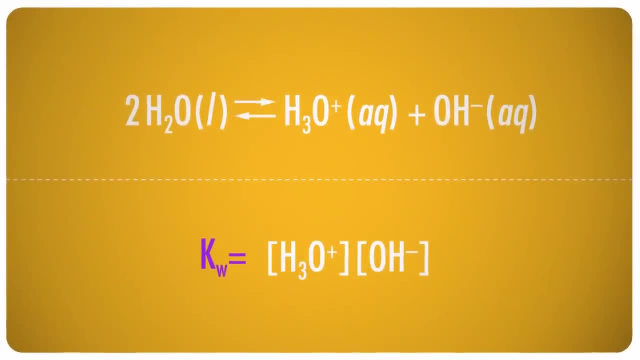 are formed in a one-to-one ratio, so their equilibrium concentrations must be equal. That means if we call the concentration of H3O+, for example, X, then the concentration of OH- must equal X as well. So the formula for the dissociation constant 1.0 times 10 to the negative 14th simplifies. 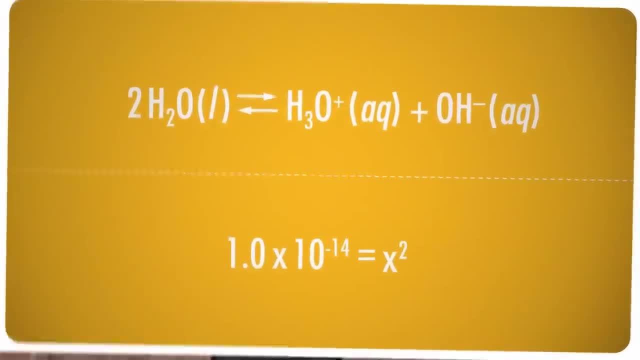 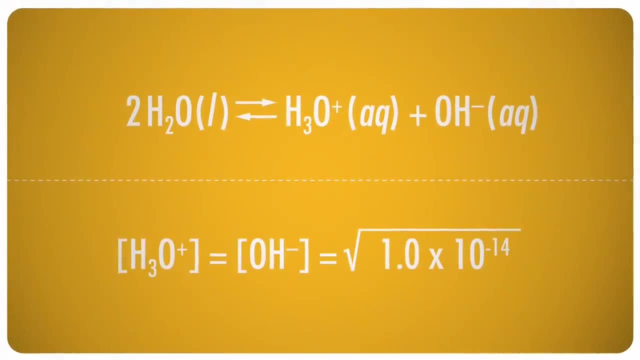 even further to X times X or X squared Suddenly. it's crazy easy. The equilibrium concentration of each ion is just the square root of 1.0 times 10 to the negative 14th. Touch one key on the old calculator and hello: both concentrations equal 1.0 times 10 to. 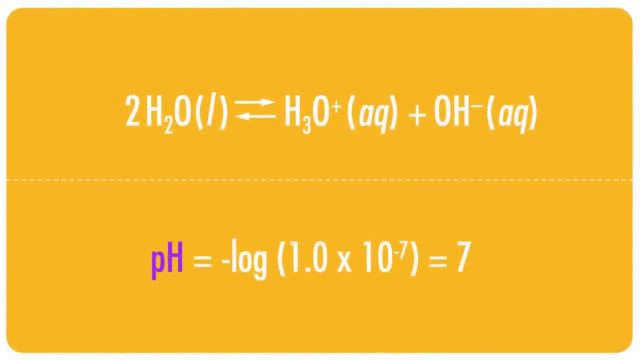 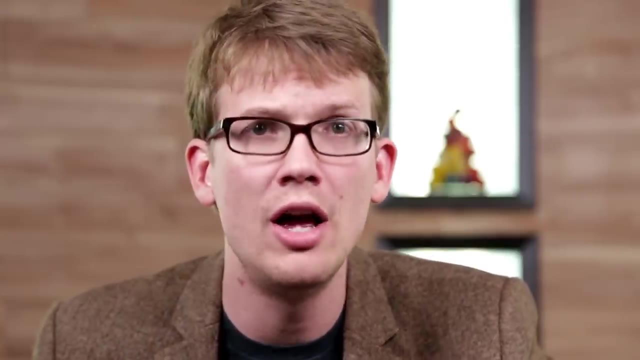 the negative 7th moles per liter at equilibrium. The pH, then, is simply the negative log of that which is 7.. This, my friends, is the basis of the pH scale. Water is neutral, so 7 is the center of the scale. 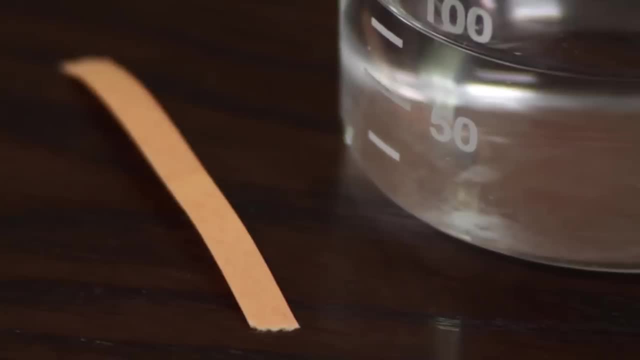 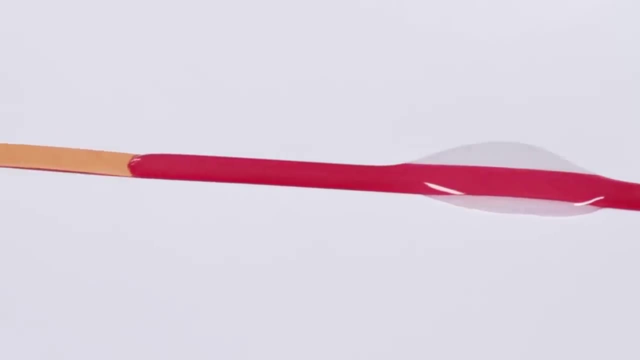 And I can prove it too. This is a strip of paper that's been infused with a chemical called litmus. Litmus is a pH indicator, a chemical that turns different colors at different pHs. There are many different indicators with many different colors, but we'll talk more about. 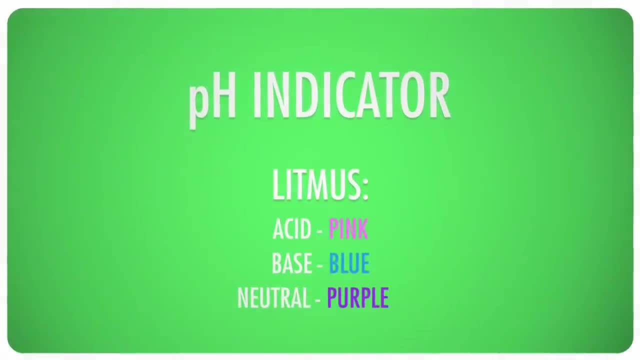 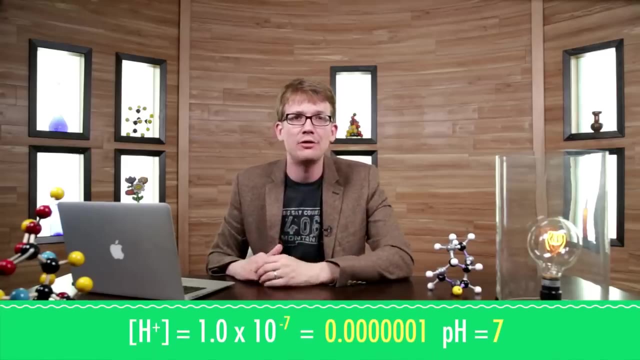 those next week. For now, just know that litmus paper turns pink in acids, blue in bases and a sort of light purple in acids. But one thing you need to remember about the pH scale: because pH is calculated from a negative logarithm, it turns everything backward. 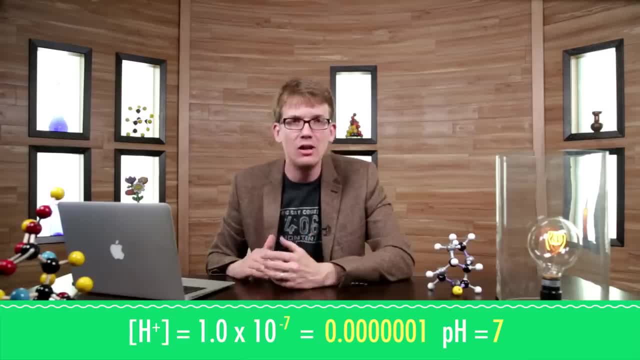 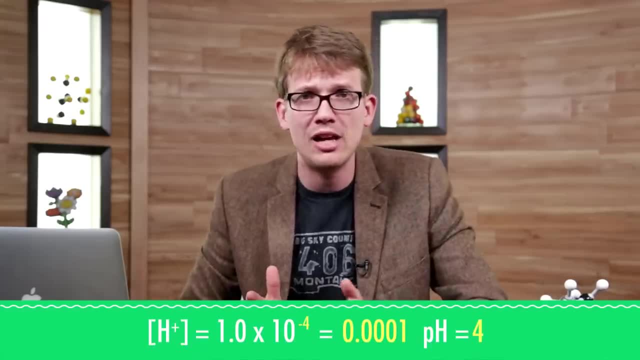 When the hydrogen ion concentration goes up, the pH gets lower. For instance, if a little acid such as vinegar were added to the water, the concentration of hydronium ion might rise to, say, 1.0 times 10, to the negative 4th moles per liter, which. 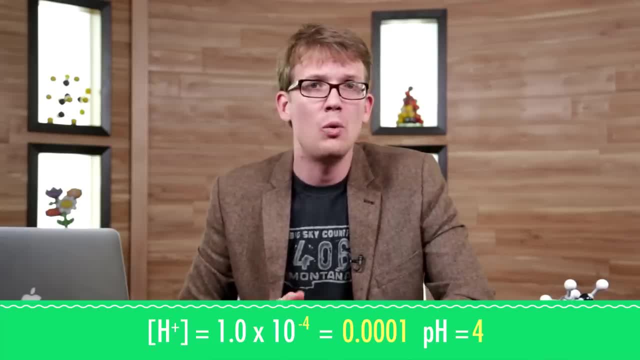 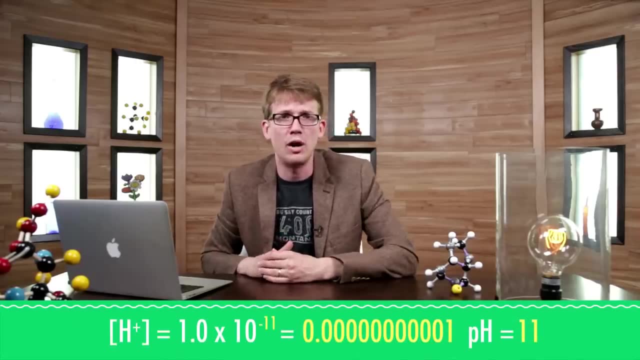 is a thousand times more than before. That concentration would push the pH down to 4.. On the other hand, a base such as ammonia would consume a lot of hydrogen Hydrogen ions if it were added to the water. If the hydrogen ion concentration drops to 1.0 times 10, to the negative 11th, a thousandth, 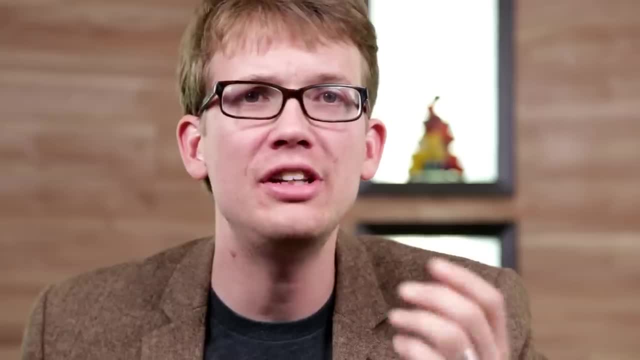 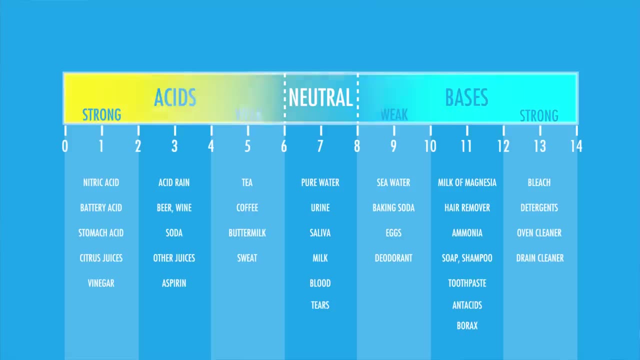 of the equilibrium concentration, the pH will be 11.. As you can see, the logs turn out to be a mathematical shorthand that saves us from dealing with very huge or very tiny numbers. The pH scale, then, is normally written from 0 to 14, with numbers below 7 representing 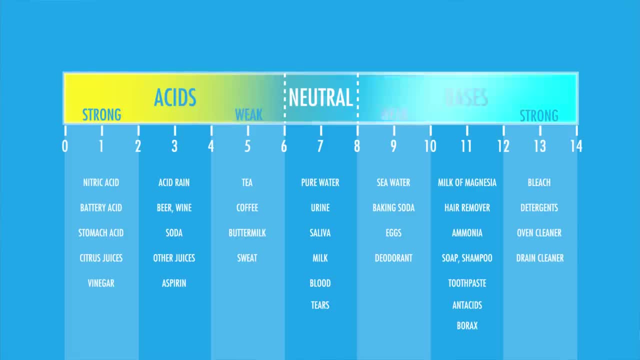 acids and numbers above 7 representing bases. It could also go below 0 or above 14, but that only happens in super-extreme conditions, in cases that you are very unlikely to encounter- at least I hope- Acids like hydrochloric or nitric acid, which ionize strongly, sometimes even completely. 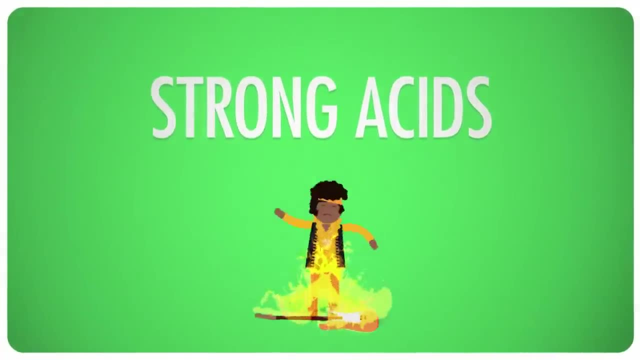 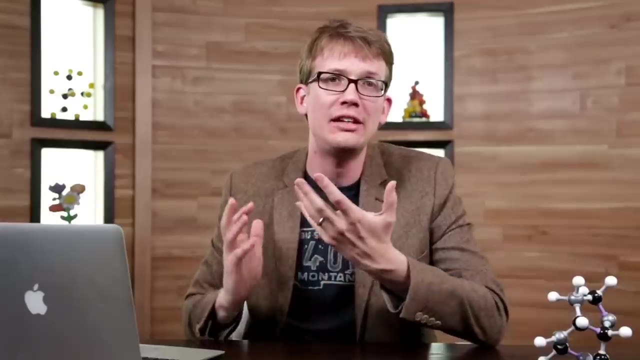 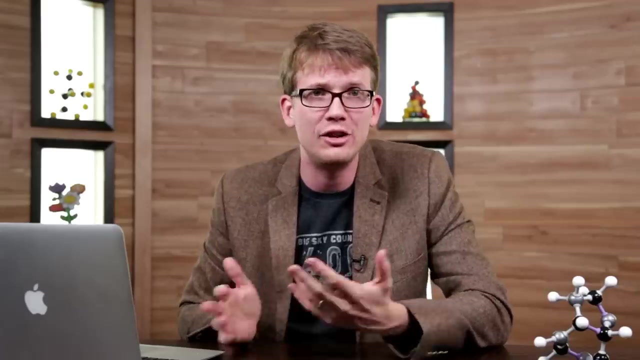 thus releasing a lot of protons, are called strong acids because they raise the hydrogen concentration a lot. They also generally have very low pHs. Weak acids like citric acid dissociate incompletely, releasing much smaller amounts of hydrogen ion, and therefore they usually have higher pHs generally considered to be in like. 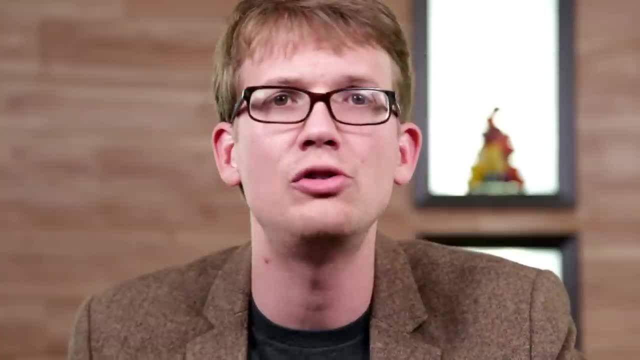 the 4 to 6 range. Strong bases, meanwhile, like sodium hydroxide, contain a lot of hydrogen ions and therefore they usually have higher pHs generally considered to be in the 4 to 6 range. Baking soda consume large amounts of hydrogen ions, leaving the concentration very low. 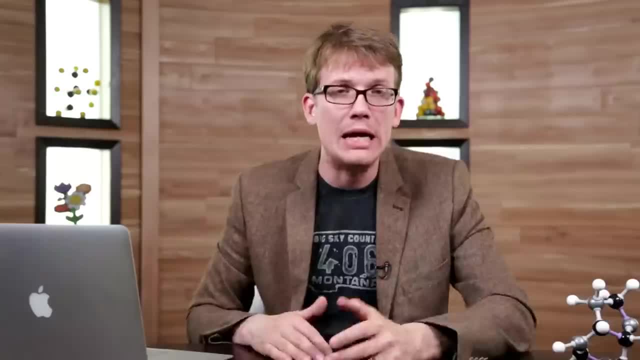 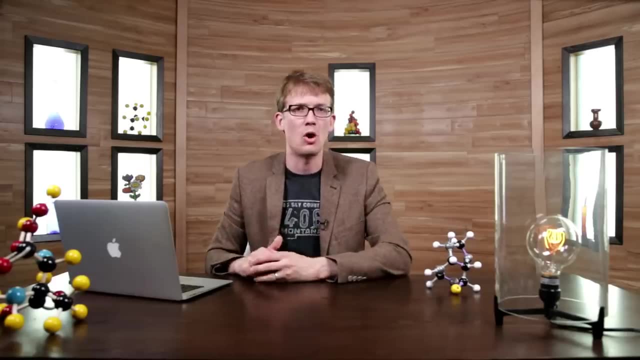 so they tend to have very high pHs. Weak bases like sodium, bicarbonate, baking soda, consume much less and generally have pHs in the 8 to 11 range. Neutral pH is technically just 7.0, but in a more practical sense it's usually considered. 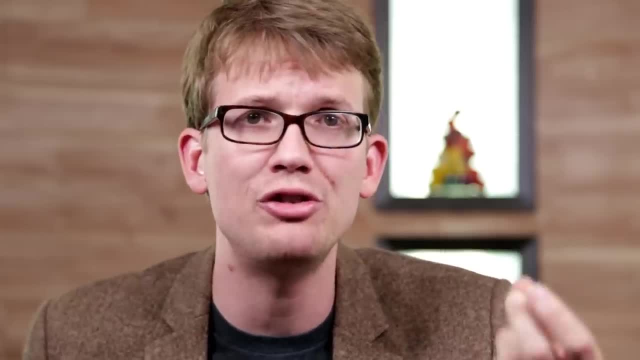 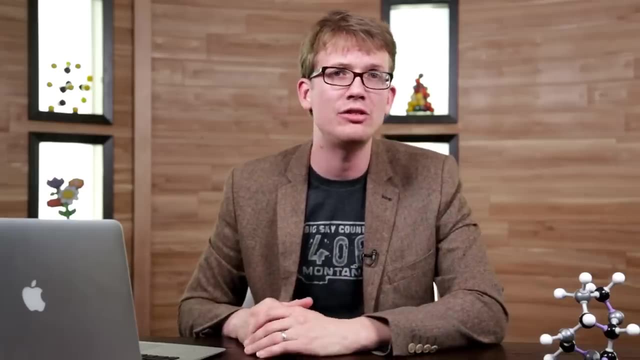 to be between 6 and 8.. So if pH is based on the concentration of hydrogen, that is, hydronium ions, what about the concentration of hydroxide ions? Just as we can calculate the pH of a substance from its hydrogen ion concentration, we can: 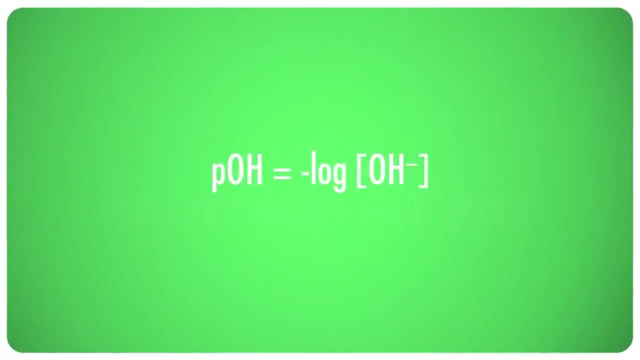 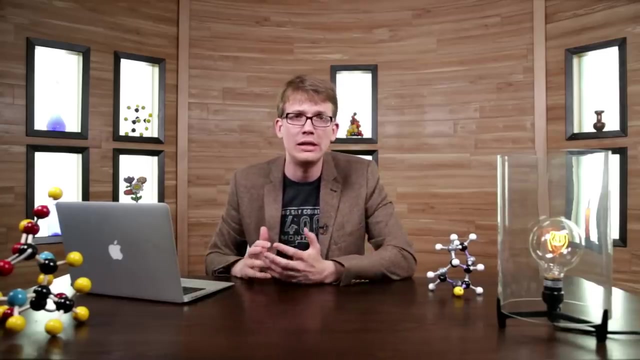 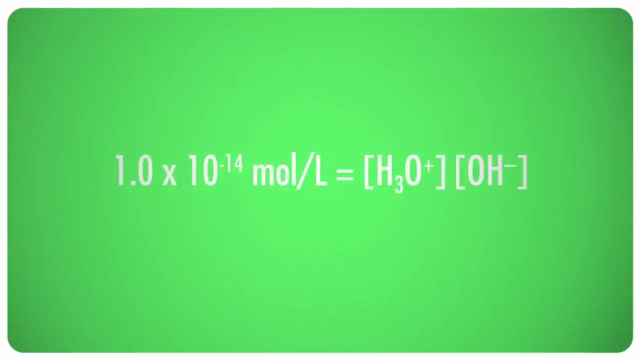 calculate the pOH, the negative log of the hydroxide concentration. This is easy because Kw never changes. Although the concentrations of hydrogen and hydroxide are only equal in pure water or perfectly neutral solutions, the product of the two concentrations always equals 1.0 times. 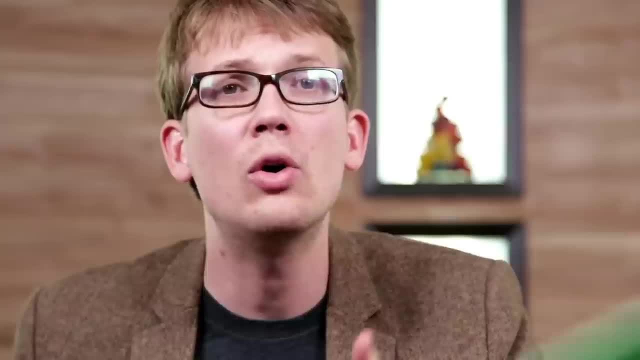 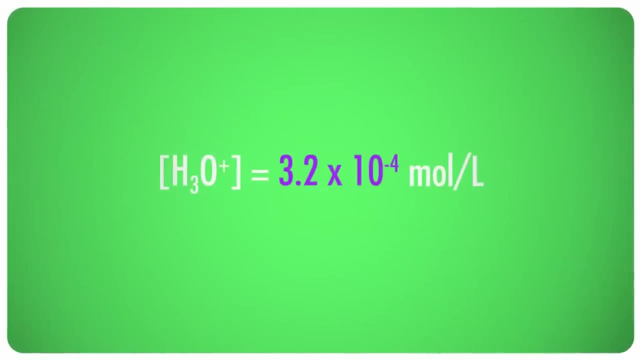 10 to the negative 14th in any aqueous solution, So like orange juice, which is really just an aqueous solution of sugar and citric acid and a few other things. say, the hydrogen ion concentration in your OJ is 3.2 times 10 to. 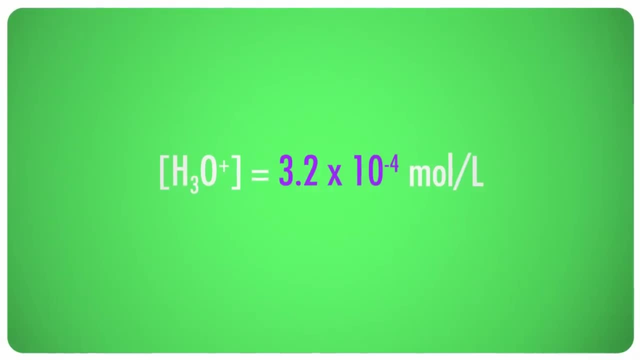 the negative 4th moles per liter. Just for the fun of it, let's go ahead and calculate what the pH is at that point, which turns out to be 3.5.. But we can also use the Kw and the hydronium ion concentration to do a very simple division. 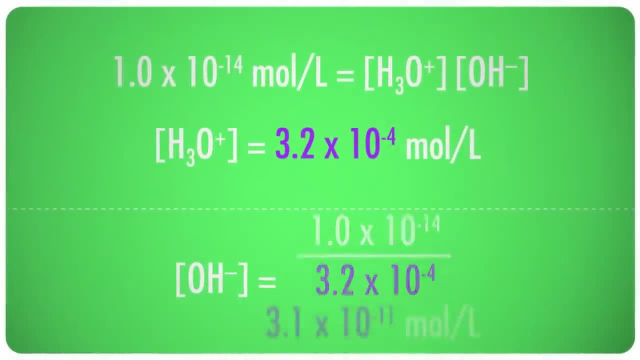 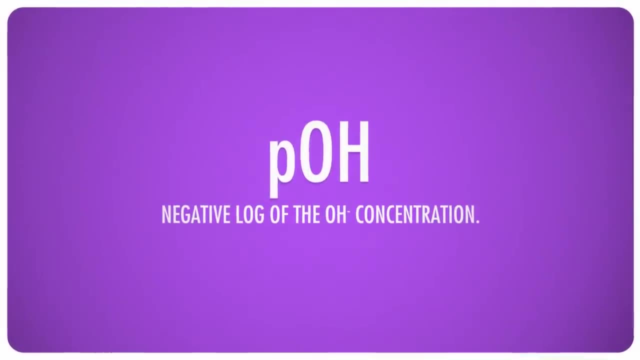 problem and find the hydroxide concentration. It works out to 3.1 times 10 to the negative 11th moles per liter. And once we have the concentration we can take another step. We can find the pOH of the solution, which is similar to the pH, simply the negative.